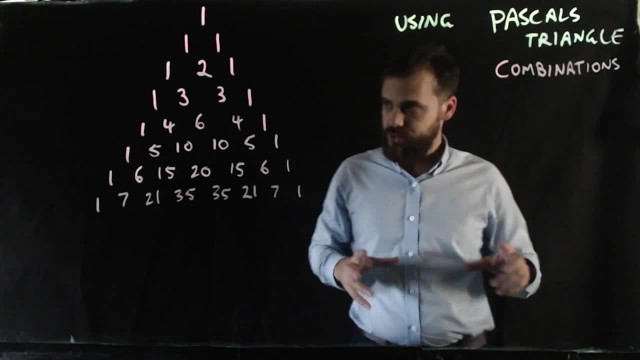 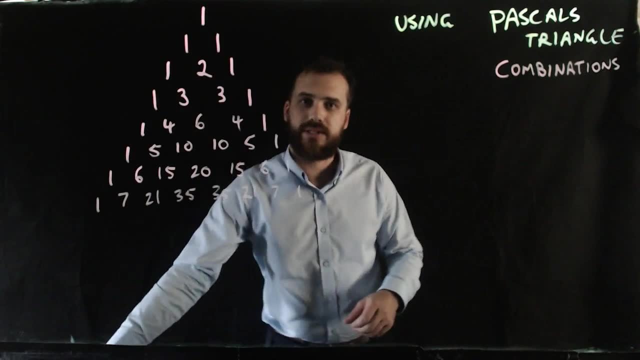 you might be a bit confused right now, but that's okay. Now, in order for us to do that first, before we even get started here, we want to label our rows. Now, key point to take away: When you're counting these rows, you start at row zero. This is 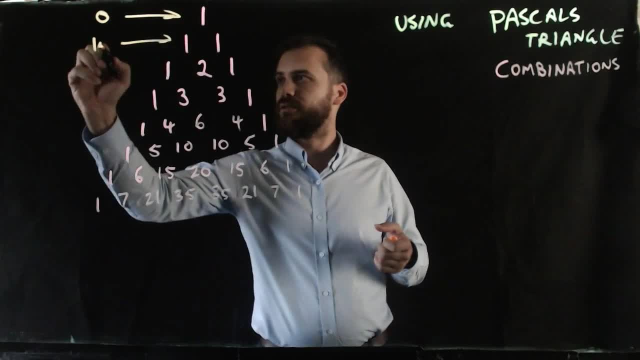 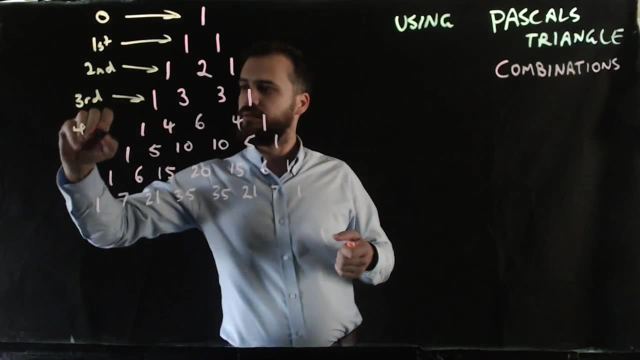 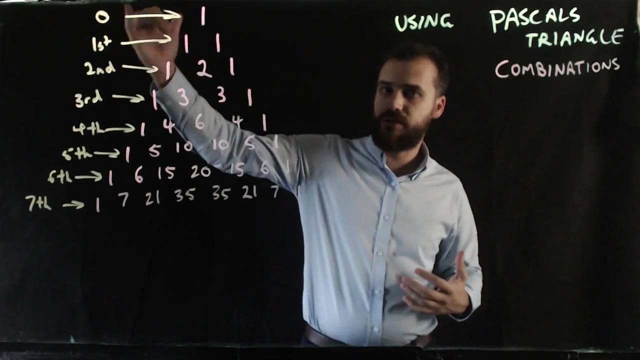 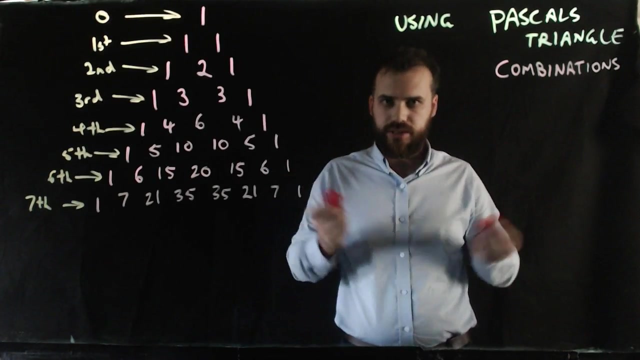 the zeroth row. This is the first row and this is the second row. You should get the idea here. Okay, so now what will this do for us? That we have the zeroth row down to the seventh row? What can we figure out? It really comes down to this Coin tossing. 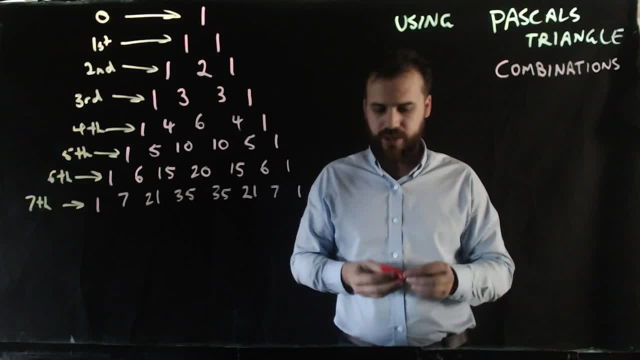 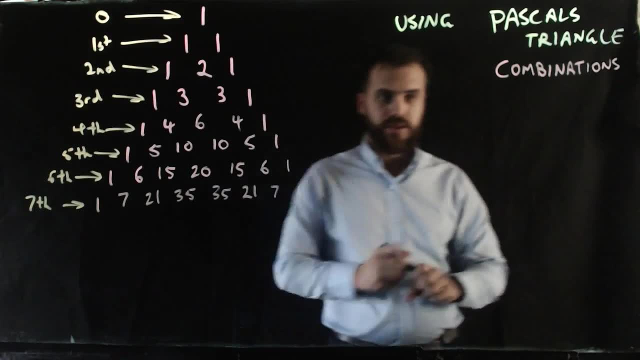 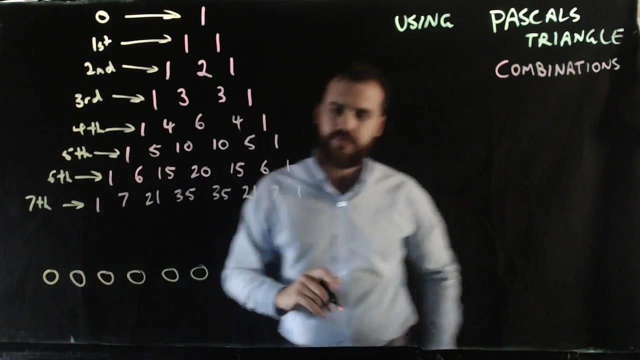 Now let's use some coins. I've got one, two, three, four, five. I've got six coins. Okay, so I'm just going to draw up six coins somewhere- One, two, three, four, five, six- And the question is: how many rows do we have? 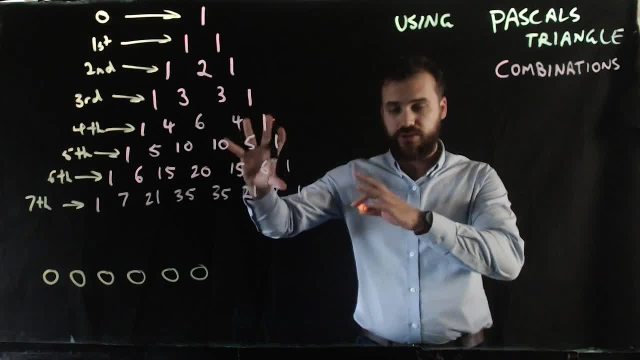 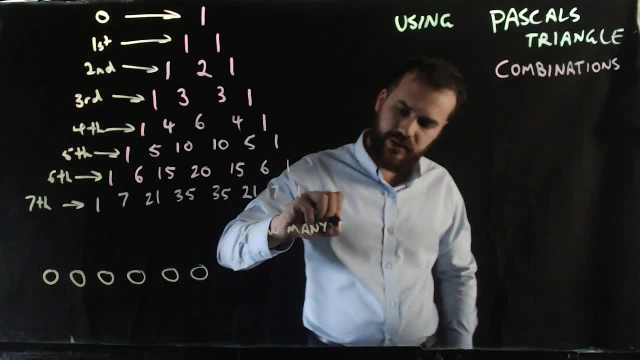 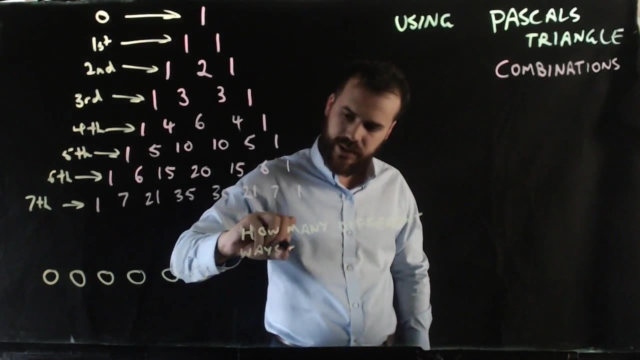 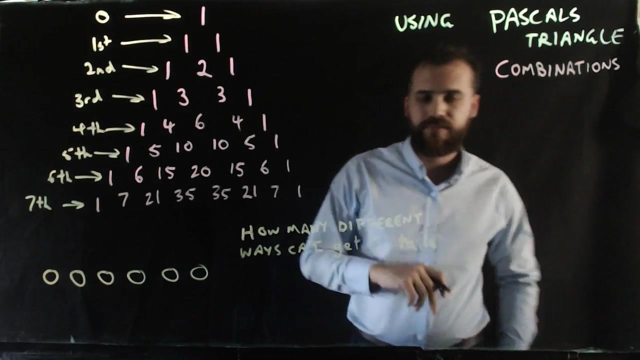 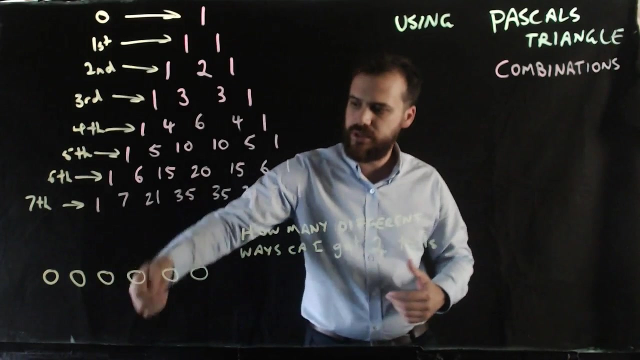 The question I can answer with my Pascal's triangle is this: How many different ways can I get two tails? Okay, that's a pretty tough question if you think about it. So what I'm going to do is toss this, This coin, toss this coin, toss this coin, this one, this one, this one And the question. 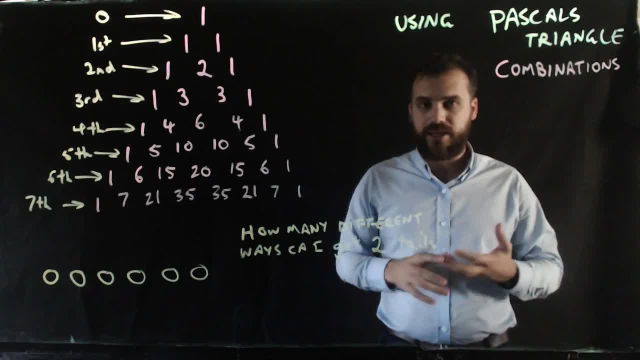 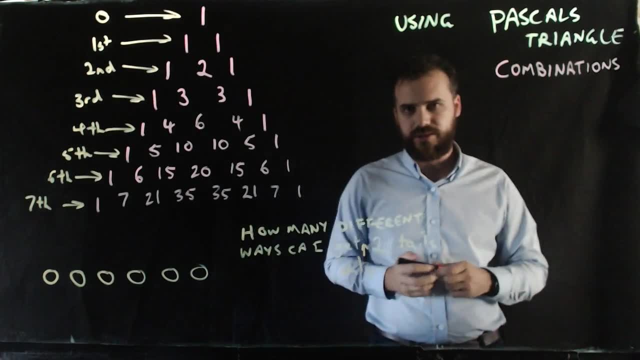 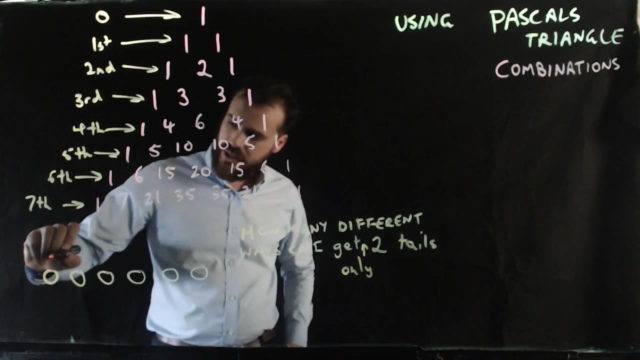 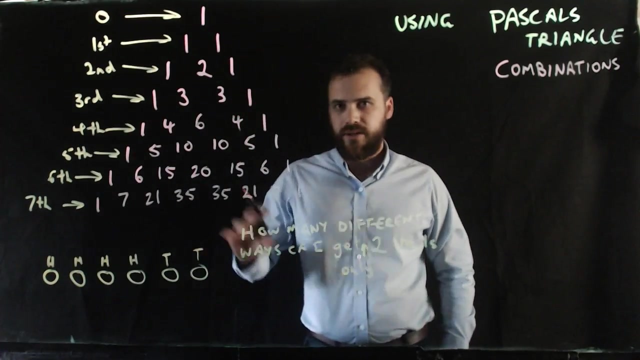 is: how many different ways could I get only two tails, Just two tails? Can I get only two tails? So it's a tough question because if you think about it, it could happen in heaps of different ways. For instance, heads, heads, heads, heads, heads, tails, tails, So tossing. 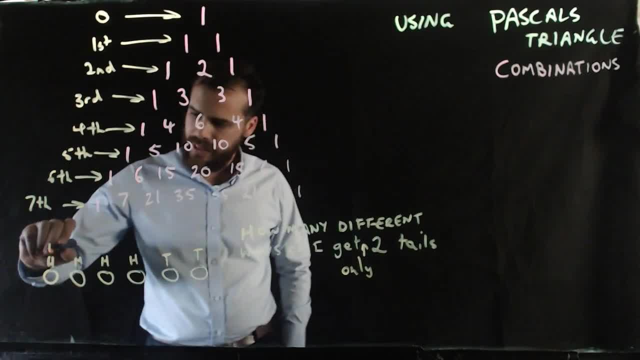 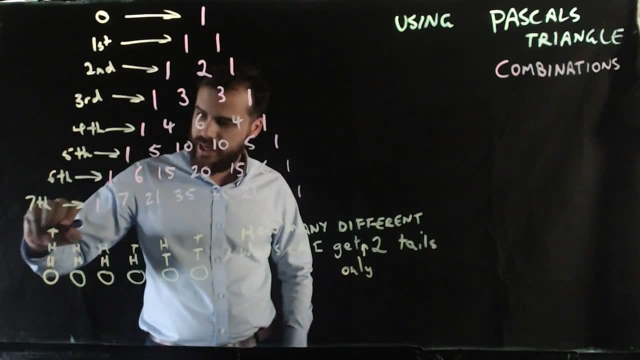 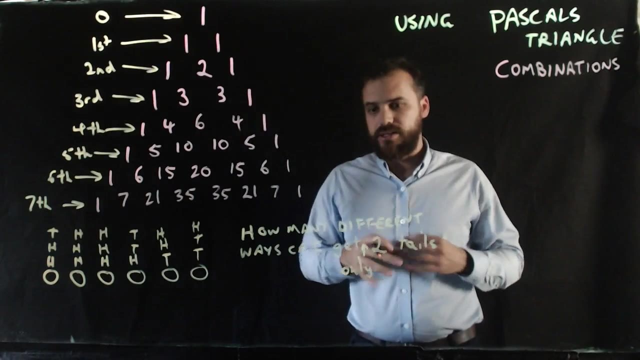 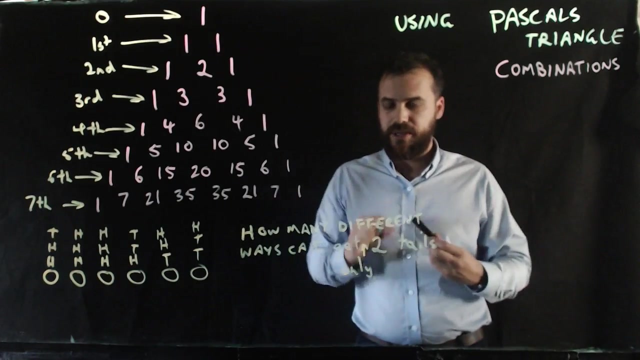 four heads and then two tails, Or it could be heads, heads, heads, tails, heads, tails Could be like that. Or it could be tails, heads, heads, tails, heads, heads. Heaps of different ways that I could get two tails. So how do I do it? Well, a bit of a step-by-step. 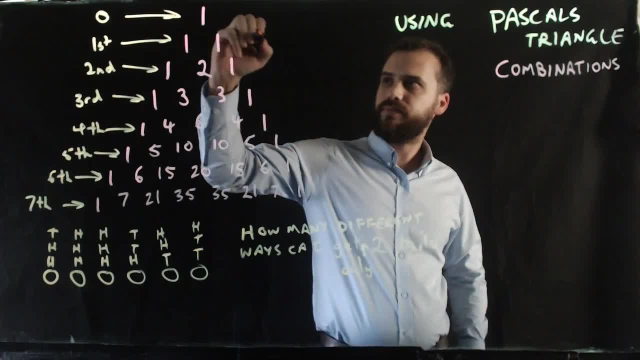 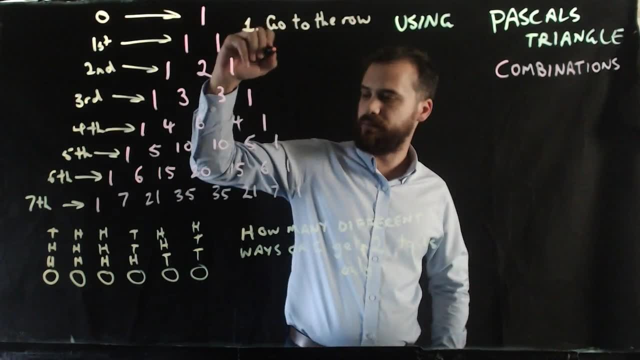 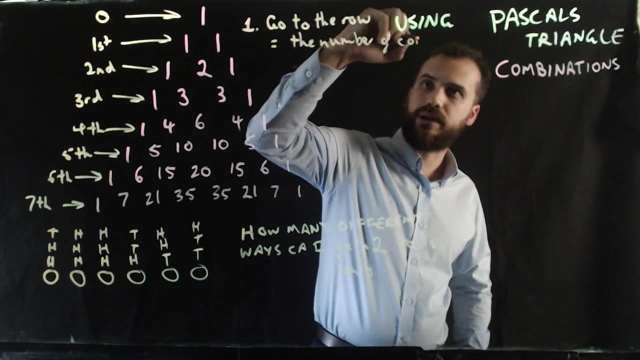 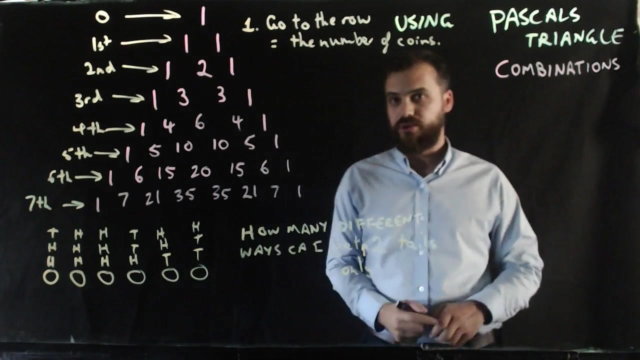 process: Step one, Step two, Step three, Step four. I go to the row equal to the number of coins. Step one Go to the row equal to the number of coins: One, two, three, four, five, six coins. So. 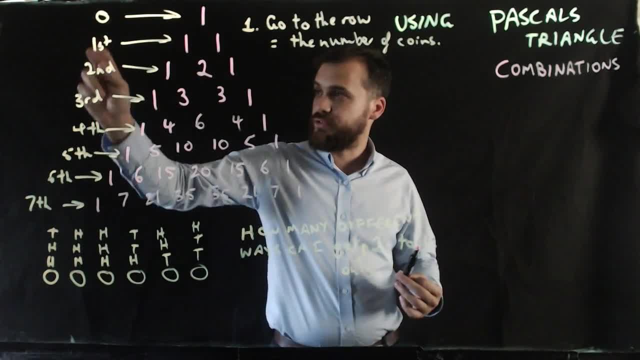 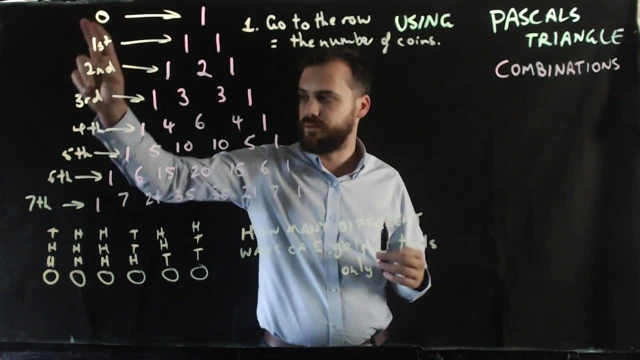 I have to go to the sixth row. Ah, First row, second row, third row, fourth row, fifth row. Now it looks like the seventh row, but remember, this is our zeroth row, So we go all the way down to our sixth row. 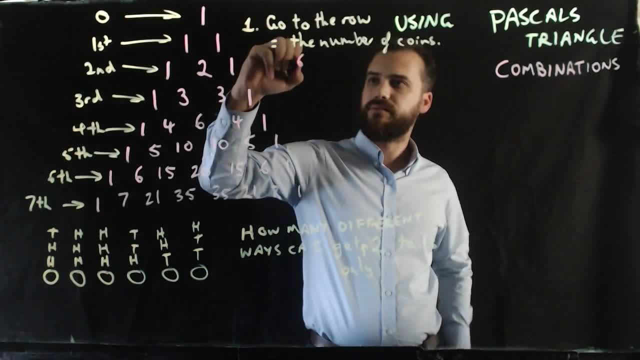 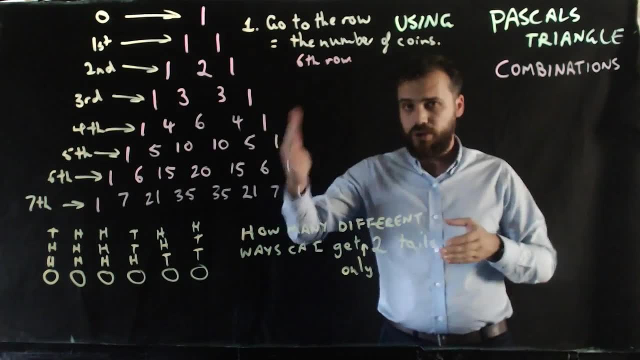 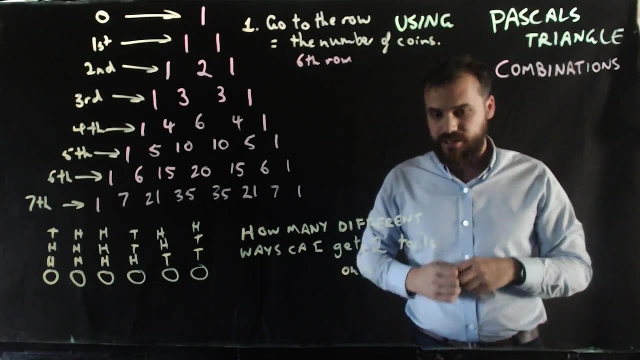 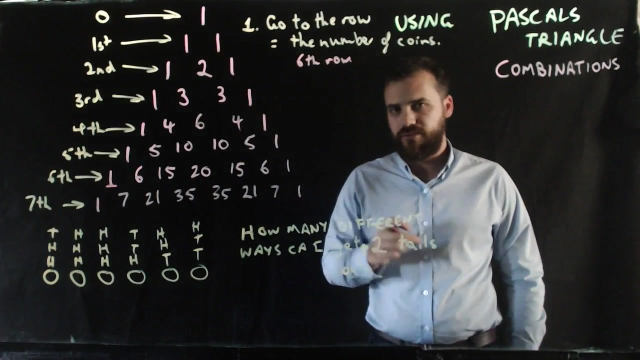 Okay, so sixth row done. Now, after I've gone down to my sixth row, we need to work across the row, And working across the row will tell us how many different ways it can happen. Now, the number one on the end represents the number of different ways that you can get zero tails. 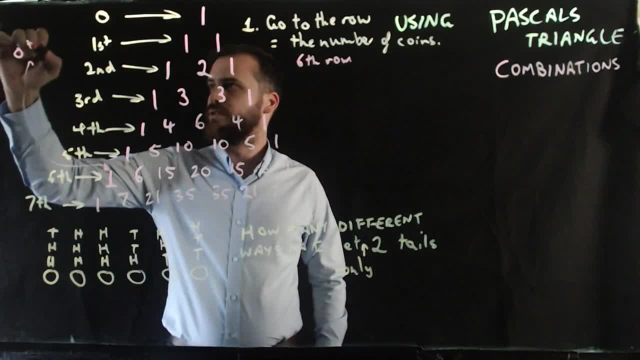 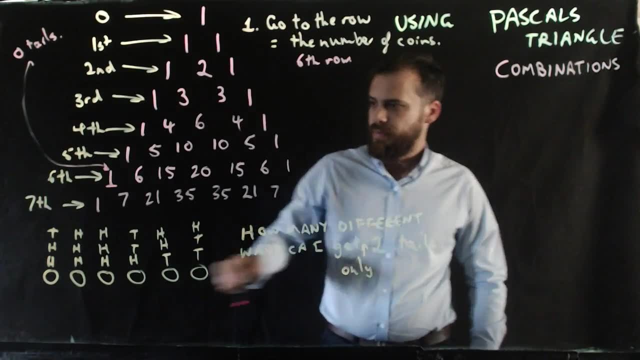 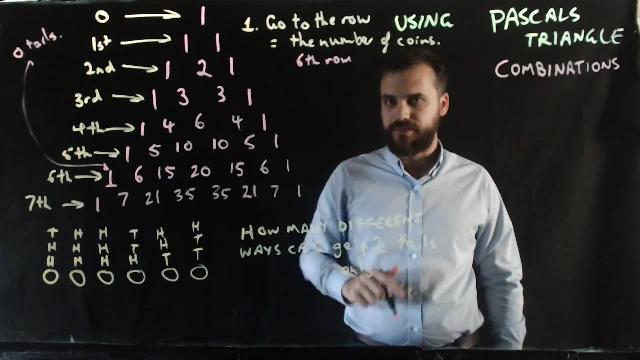 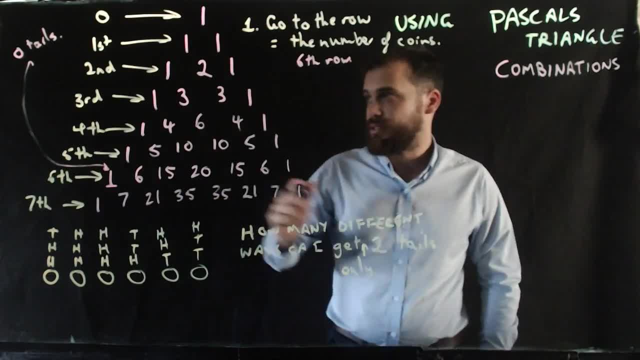 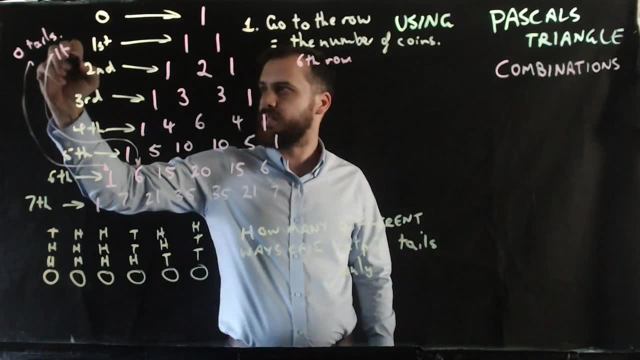 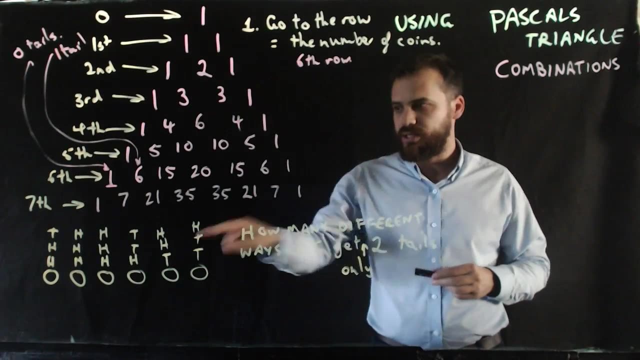 Now our second number here. the number six represents the number of different ways that you can get one tail. Now that makes sense as well. There are only six different ways that you can get one tail here. One way is to toss tail, followed by five heads. 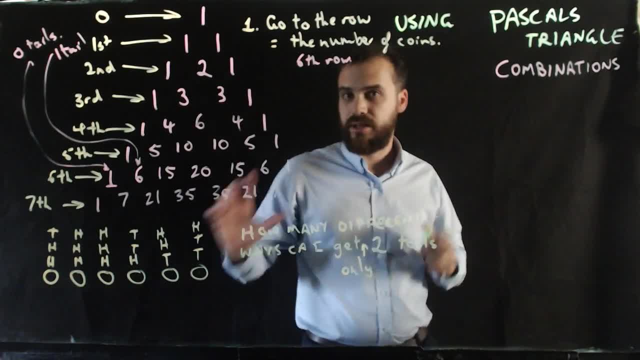 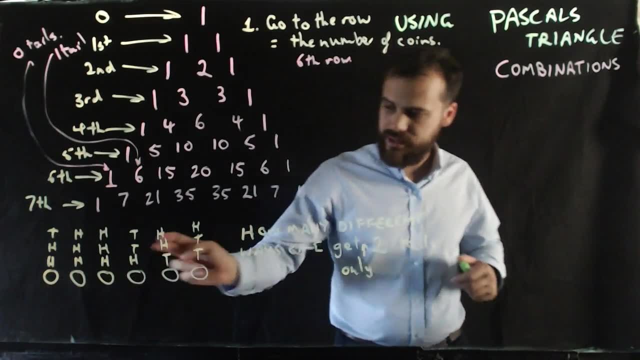 Or the second way would be: heads tails heads, heads, heads, heads. The other way would be heads, heads, tails heads, heads, heads, Heads, heads, tails, heads, heads, heads, heads, heads, tails heads and heads, heads, heads, heads, heads tails.